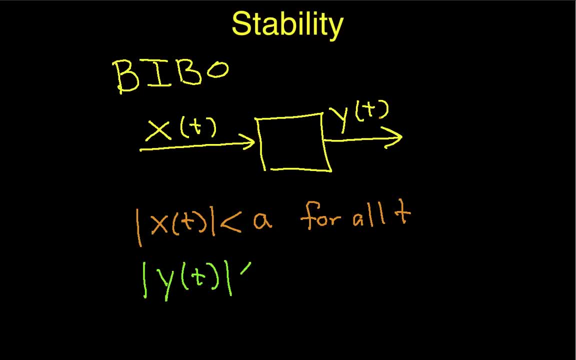 output will be less than b for all t. So if this statement implies that this statement is true, then the system is- bounded input, bounded output- stable. Conceptually, what this means is that as long as the input does not get to be too large, so as long as this stays bounded, then the output stays bounded. 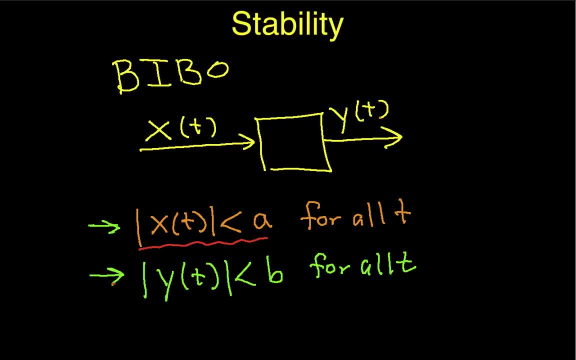 and the idea is that that usually means that the system's stable. Well, that means that the system does what you want it to do, or at least doesn't do what you don't want it to do. So let's do a few simple examples of systems and try to determine. 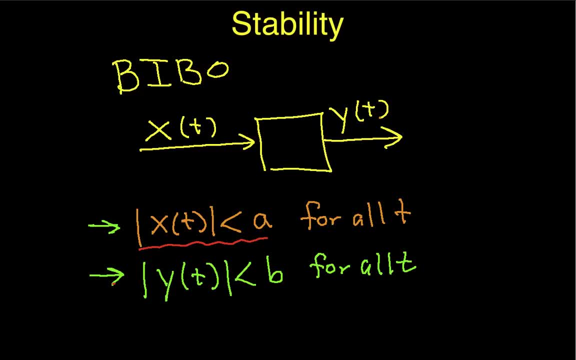 if they're unbounded, or unbounded BIBO, stable. So suppose we have a system where what the system does is multiply the input by a gain, so that y of t is equal to some gain times x of t. And the question is: 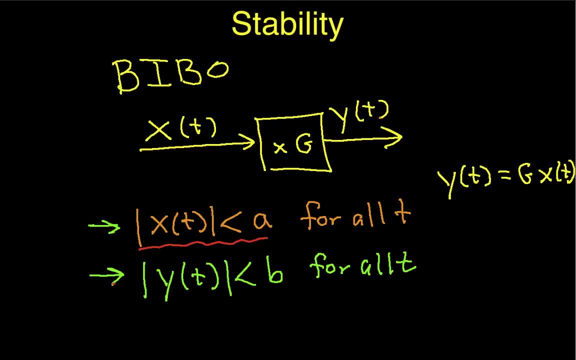 is this a bounded input, bounded output, stable system? Okay, well, the idea, or we have to check that if this is true, that is, if x of t, the magnitude of x of t or the absolute value of x of t is less than a, then will the mag or the 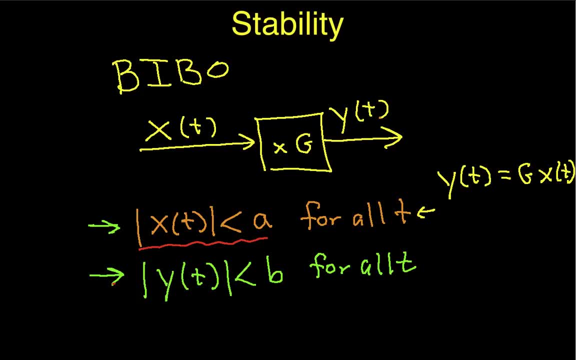 absolute value of y of t be less than b? a. here is something that we can tell basically from the signal. So, for example, if I talk about a unit step function, where, let's say, the unit step function looks something like this: It's zero. It's zero for values of. 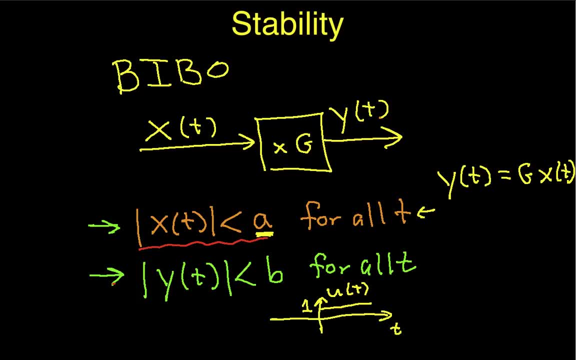 t less than zero and it's one for values of t greater than zero. Then say I pick a equals two. Well, if a is equal to two, then clearly the absolute value of u of t is either zero when t is less than zero, or one when t is greater than or equal to. 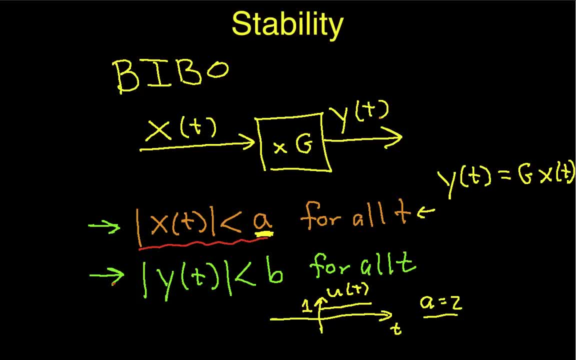 zero. So I could pick a value of a is equal to two and this inequality here would be satisfied. Okay, So let's assume that we have some arbitrary input- x of t, or this inequality is satisfied for some value of a. Now, if I look at the output, the absolute. 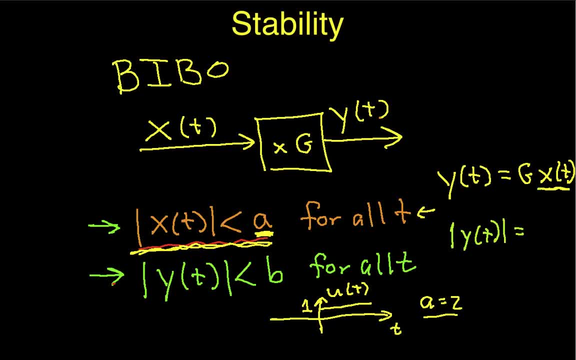 value of y of t is the absolute value of the gain times x of t, and this is the absolute value of the gain times, the absolute value of x of t, and this is less than the absolute value of the gain times a of t because, again, we're assuming that x of t satisfies this inequality. 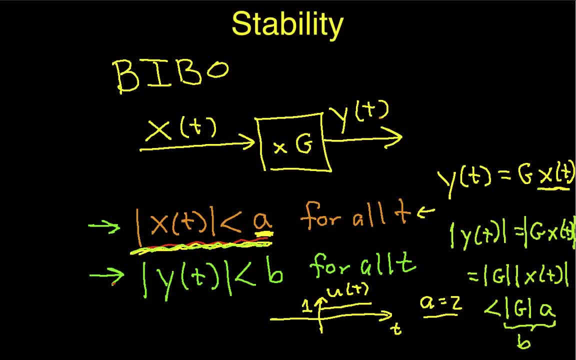 And so if we take then b, as defined by the absolute value of the gain times a, then the output of this system satisfies this inequality. Okay, So again is a biblostable system in the sense that anything, any time I put a bounded signal in, I get a bounded signal. 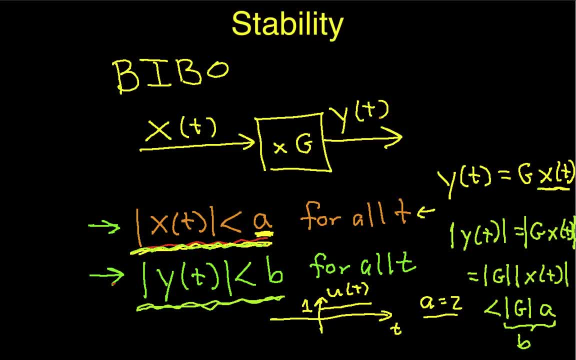 out. Okay, it is possible to have an unbounded signal, For example. well, u of t is a bounded signal. If I had e to the a? t, as t gets large, this thing gets large too, And so this e to the a? t does not satisfy this inequality here. 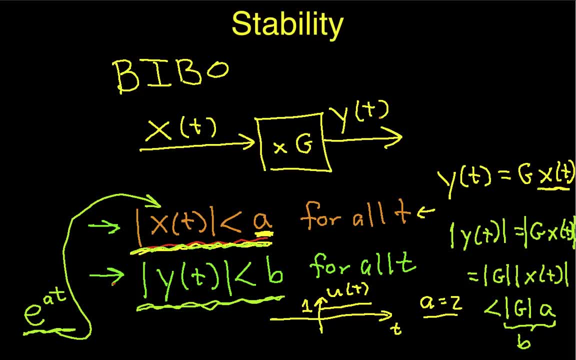 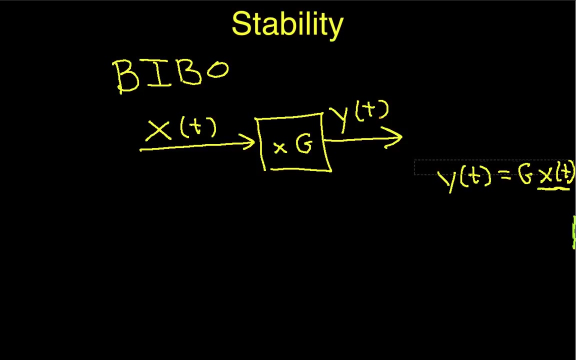 Okay. So let's look at another example. First, let's tidy up a bit, Get rid of all this clutter. In fact, we'll get rid of all of this, So we have lots of room for this next system, because it could get a little hairy. 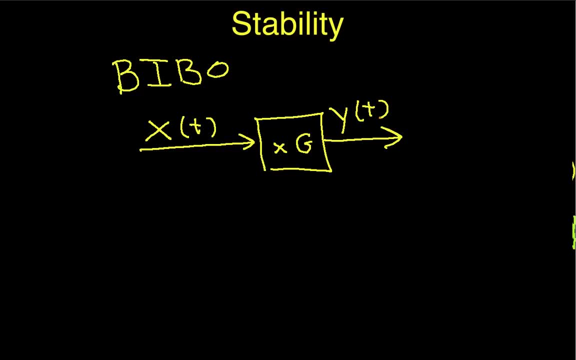 Okay. so let's suppose we have a system where the output, the input of the system, y of t is the integral from time 0 to t of the input. So we'll say x of tau, where tau is a dummy variable of integration. 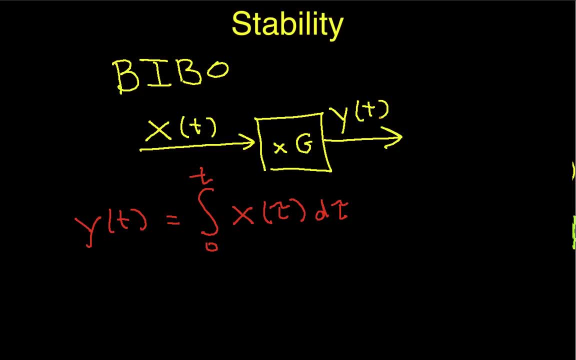 Okay, So conceptually, what this system does is, if I can graph my input, x of t, whatever it is. so this is x of t. Actually, we'll call this x of tau, since we're doing a dummy variable of integration here. 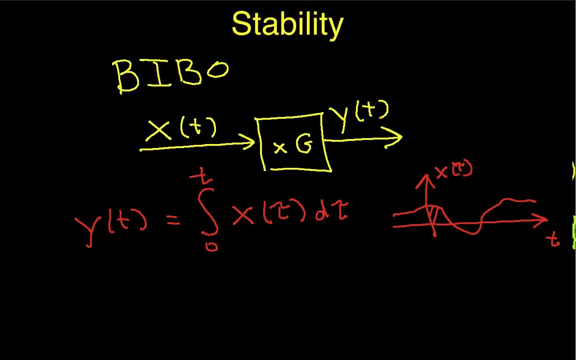 What this system does is it computes the area under x from time 0 up to some specified value of time t. Okay, So basically, the output of the system at any given time is the area area between time 0 and time t. So at a later time the output of this system is going to: 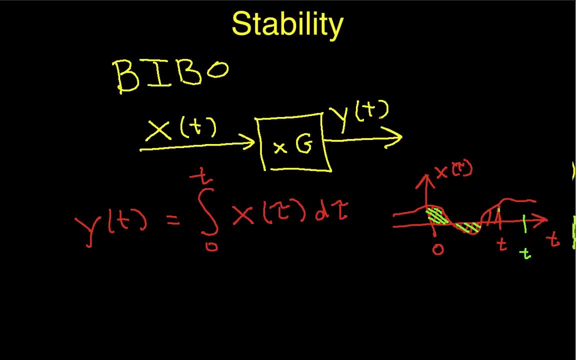 be the area under the input signal. at this later time We could call that t prime. So again, the area here, or the output, is the area from 0 to t. So is this system- bounded input, bounded output- stable? And the answer is it turns out no. The way we can show this? 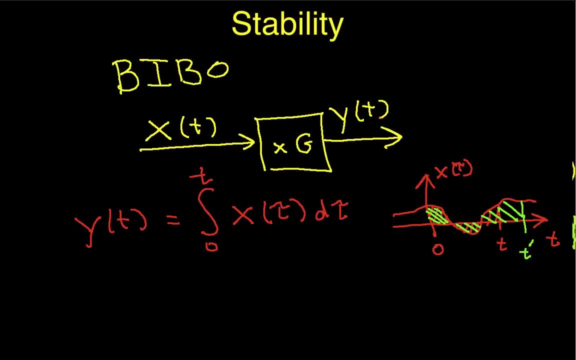 to show that a system is not bounded input, bounded output, stable. we just have to find one input that's bounded, that gives an unbounded output. So suppose that the input is the unit step function. okay, As we talked about before, this is a bounded function, So I can choose. 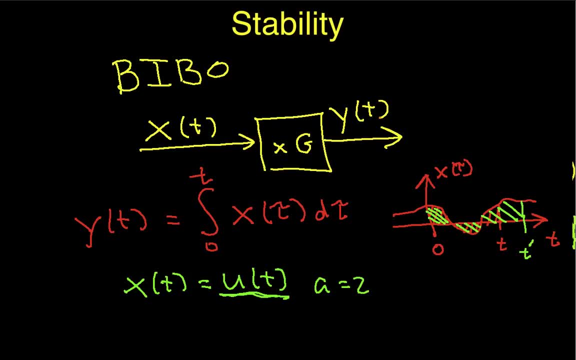 a equals 2, or I can choose a anything bigger than 1, and this is satisfied. So if I put this input into the system, the output's going to be the integral from 0 to t of this input. okay, So y of t is going to be the integral from 0 to t of um. the unit step function. 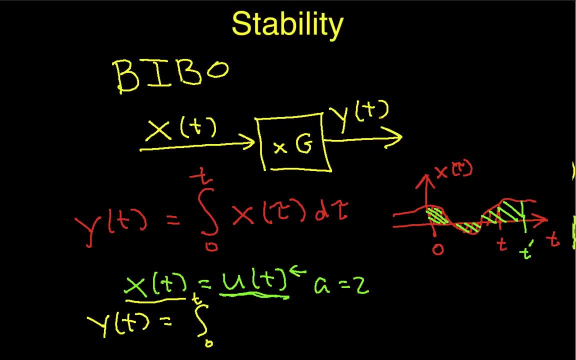 And as long as t is greater than 0, that's going to be 1.. And you can work out this integral: that y of t is now equal to t. okay, And again, this is for the case where t is greater than.